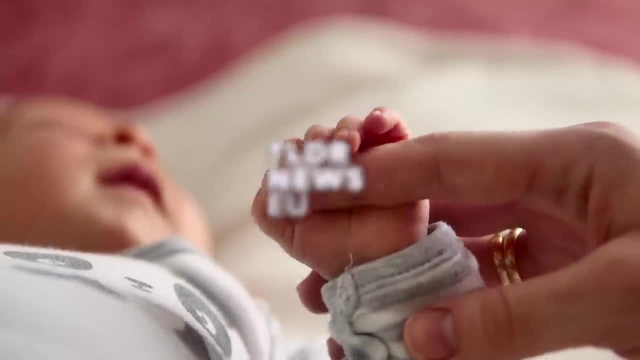 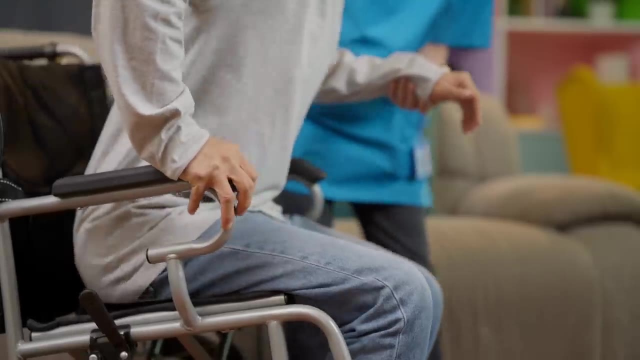 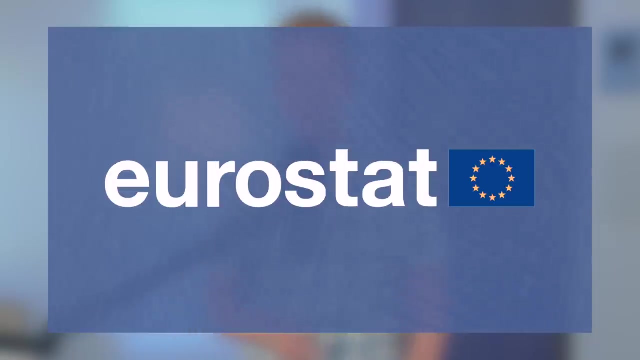 This video is brought to you by Nebula. As you probably already know, much of the world is suffering through a demographic crisis. Fertility rates are falling, putting more pressure on public services and straining national budgets. Europe is no exception, According to the latest Eurostat. 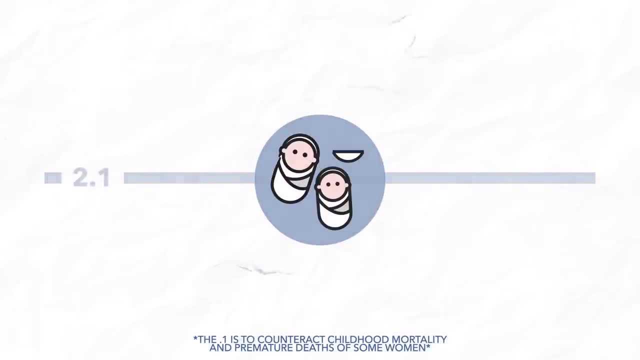 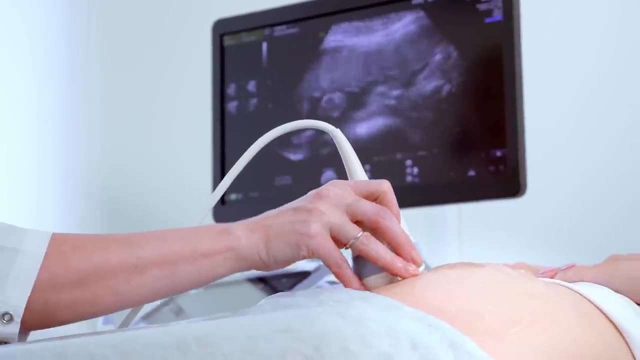 data, the EU's fertility rate was about 1.53 in 2021, well below the so-called replacement rate of 2.1.. However, provisional data for 2022 and 2023 suggest that Europe's fertility rate is now. 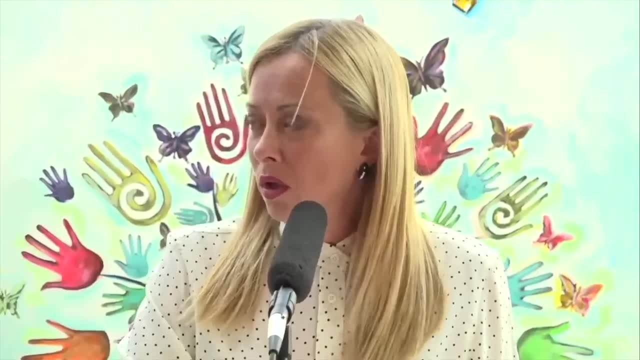 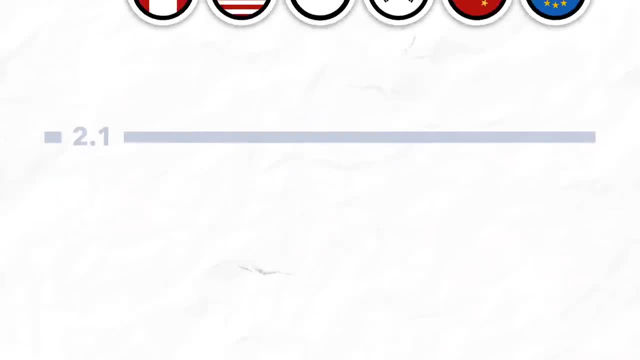 falling at an unprecedented rate and European governments are getting increasingly anxious about their demographic declines. So in this video, we're going to have a look at Europe's pre-existing demographic crisis, why it's gotten way worse in the last year or so. 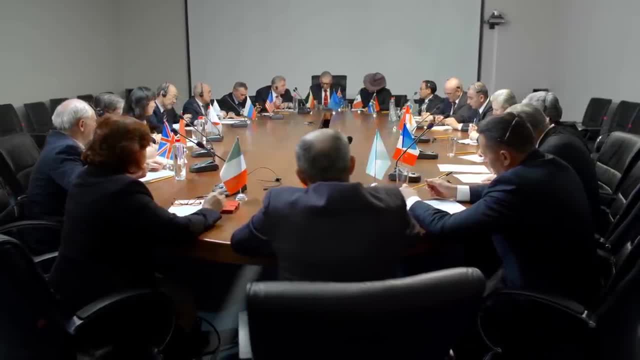 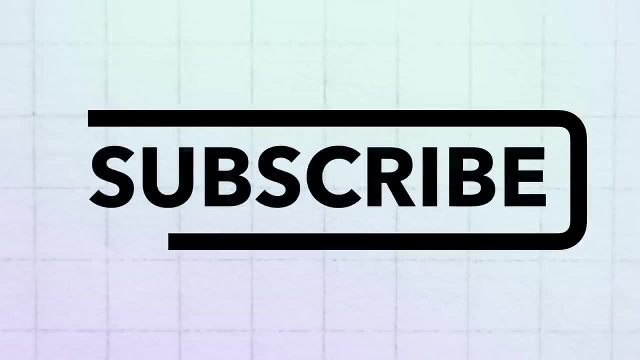 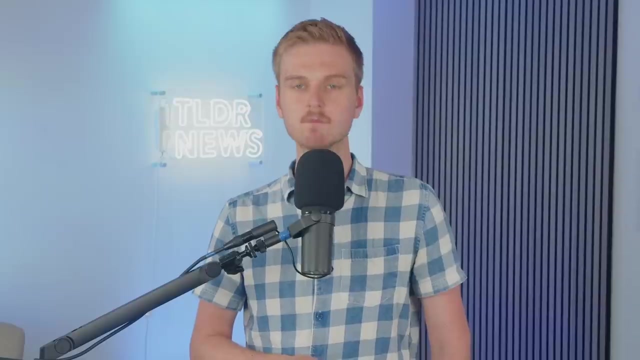 and whether there's anything European governments can do to fix it. Before we start. if you haven't already, please consider subscribing and ringing the bell to stay in the loop and be notified when we release new videos. So to understand this video you're going. 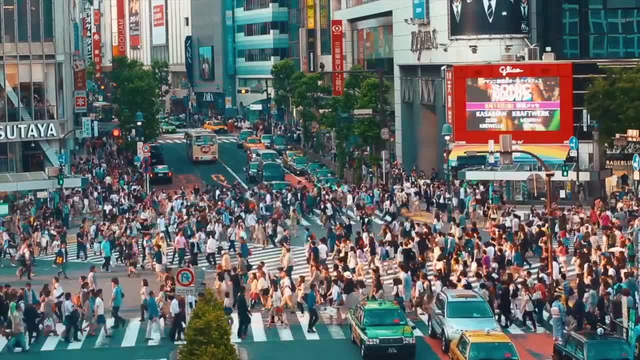 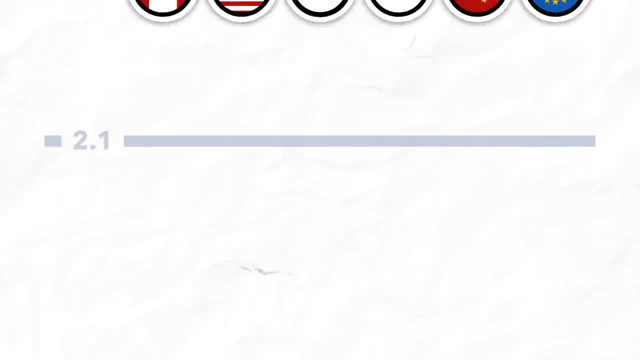 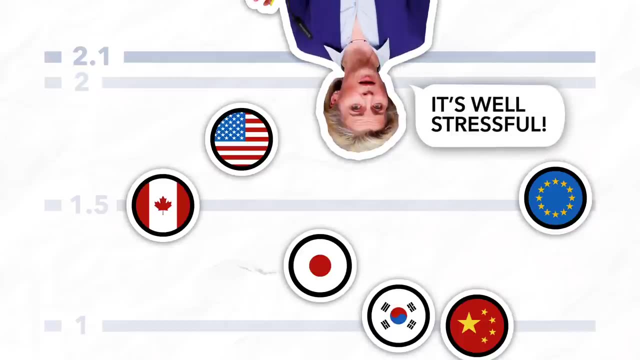 to need a bit of context. To maintain a stable population, a country needs a fertility rate that is the number of births per female of 2.1.. Low fertility rates- that is, a fertility rate significantly below the replacement rate of 2.1, are economically and politically stressful. 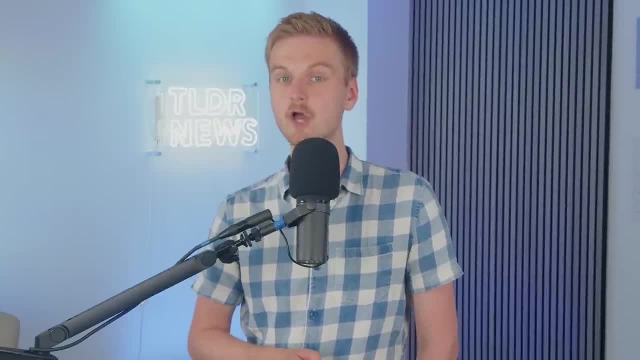 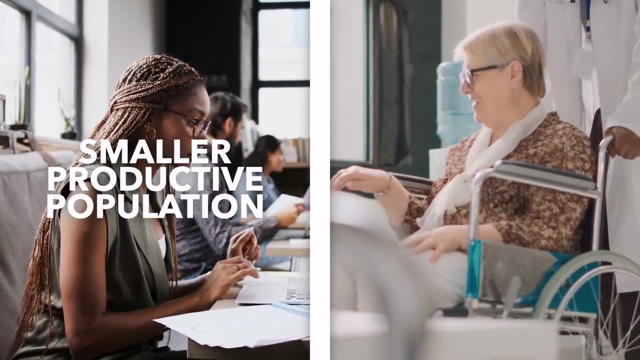 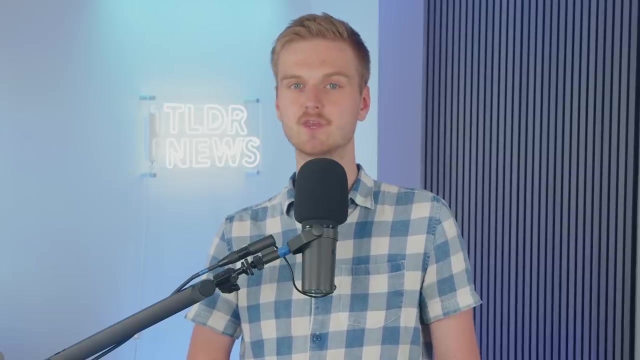 Low fertility rates mean a smaller and, importantly, an older population. This means there'll be less people of working age relative to pensioners, which means a smaller economically productive population sustaining a relatively larger non-productive population. This means two things: One, a smaller economy overall because you've got fewer working age people, and two: 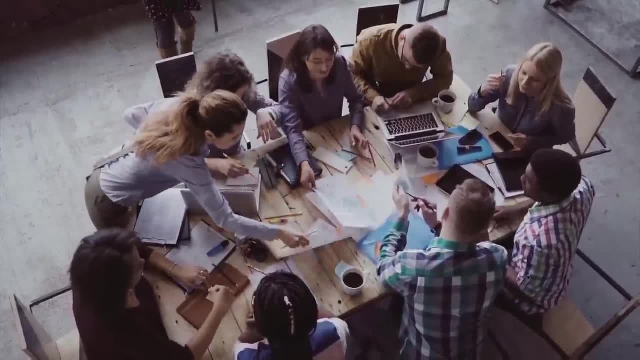 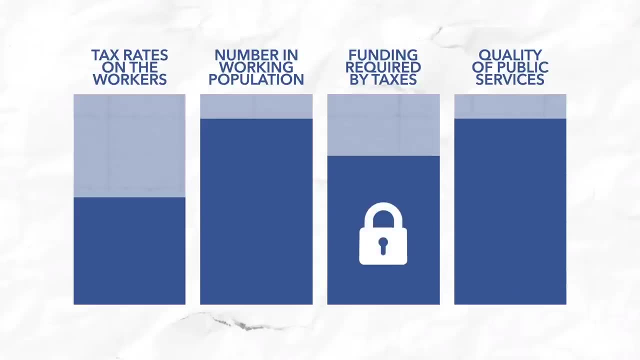 a higher tax burden on those young people that are working. This is because, assuming you want to maintain your current quality of life, you're going to have to maintain your current quality of public services. you need to make sure you're getting the same amount of tax per capita. But if 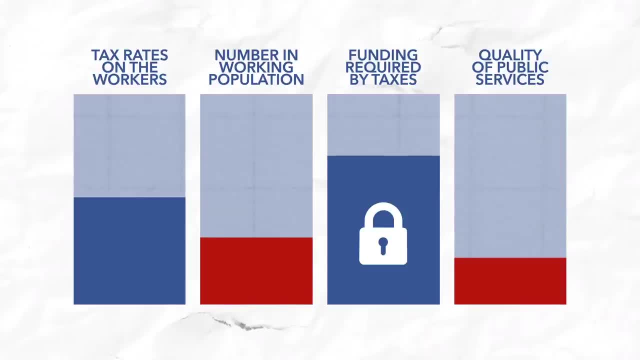 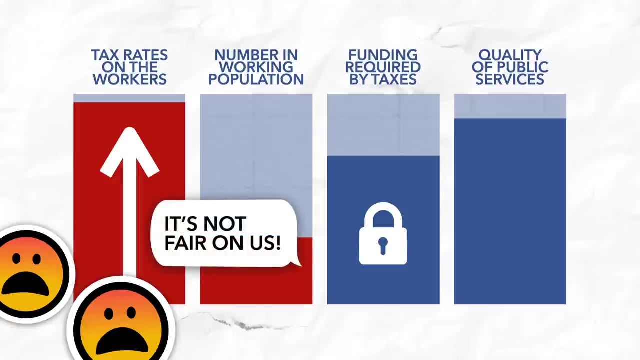 you've got fewer working age people and more idle pensioners, then you need to tax those working age people more heavily to keep standards up. This is both bad economically- a higher tax burden will, at least in theory, discourage working- and bad socially, because it creates intergenerational 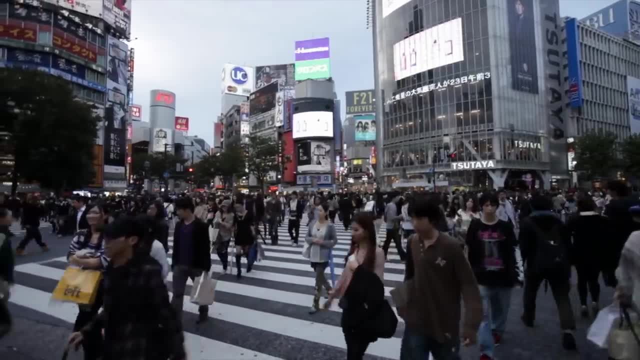 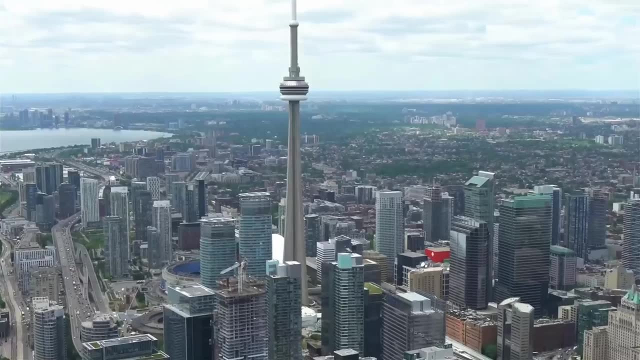 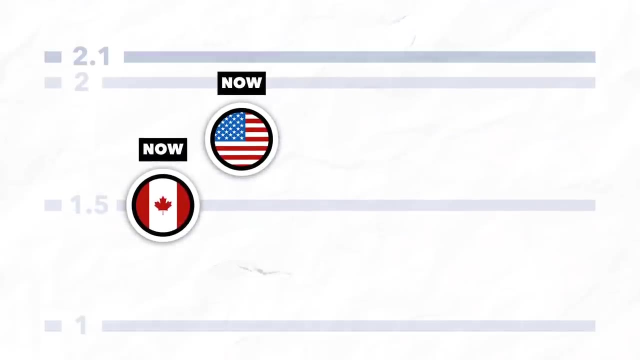 unfairness. Most of the developed world, and actually quite a lot of the developing world, is struggling with low fertility rates. The US and Canada, for example, have both seen their fertility rates fall from about 4 in 1960 to about 1.8 and 1.5 respectively today, And lots of countries in Southeast Asia, including perhaps most notably, China, have fertility rates even lower. The latest data from China, for example, implies a fertility rate of 1.09, which is pretty insane, especially when you consider that China had a fertility rate of about 6,. 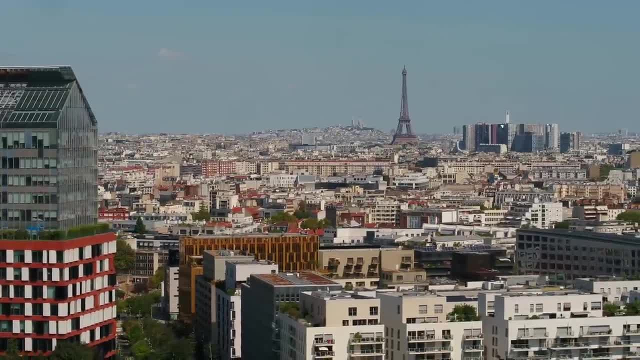 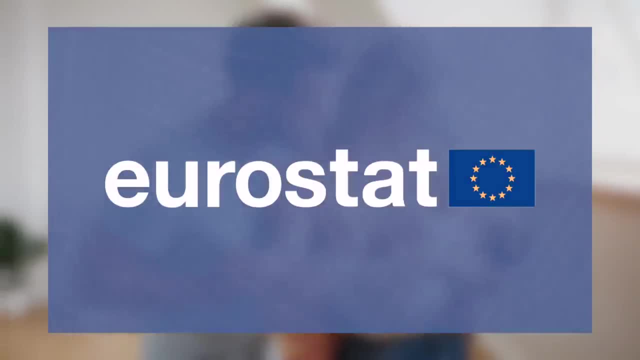 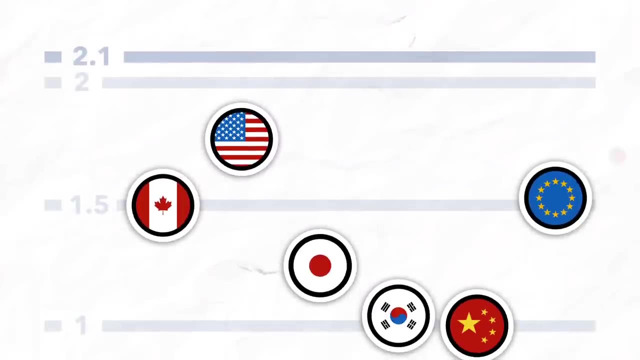 in the 1960s. Anyway, like everyone else, Europe is also struggling with a below replacement fertility rate. According to the latest Eurostat data, which runs until 2021,, the European Union's average fertility rate was 1.53, which is slightly higher than what it was in 2020, during the 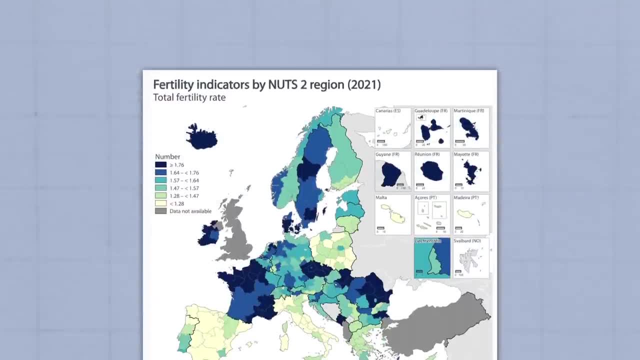 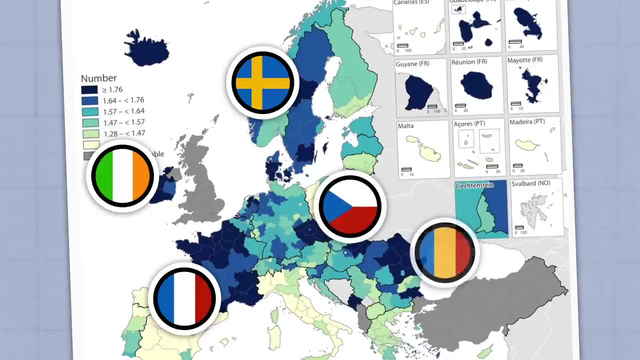 pandemic when it fell to 1.5.. The countries with the lowest fertility rates are Spain, Italy and Poland, while the highest fertility rates are in Sweden, France, Ireland and parts of Central and Eastern Europe. Now, this might not sound too bad. After all, it's somewhere between 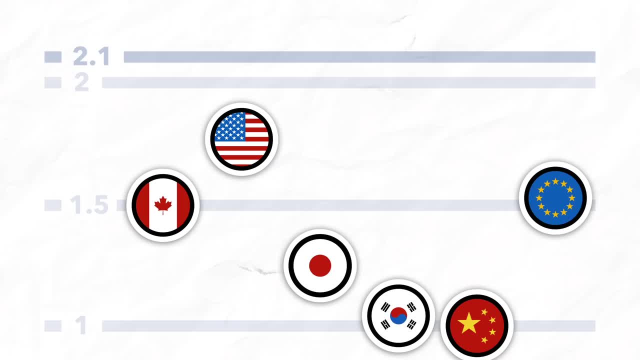 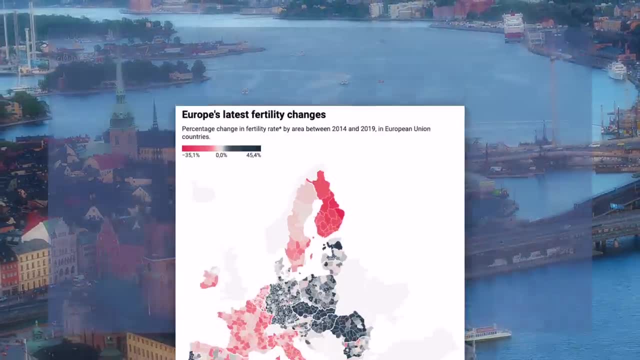 Canada and the US, and well above places like China and Japan. However, the continent-wide data masks the stark decline in certain European countries, which have been offset by increases in fertility in Central and Eastern Europe. There's an interesting divide in Europe here. 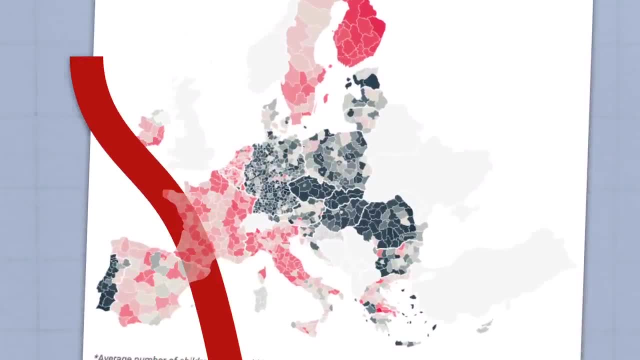 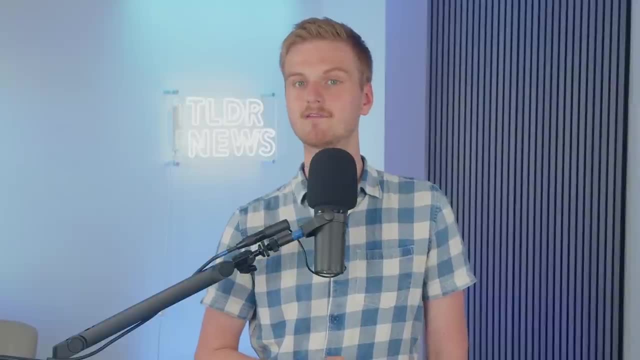 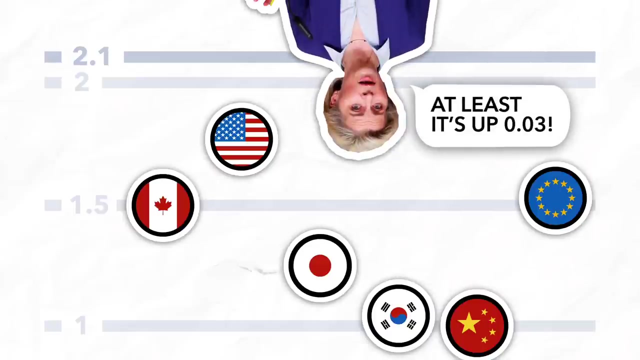 As the graph shows, fertility rates are falling across Northern and Western Europe, but actually rising in Central and Eastern Europe as well as Portugal. But, perhaps more worryingly, provisional data for 2022 and 2023 suggest that the increase in 2021 was mainly because fertility was artificially suppressed. 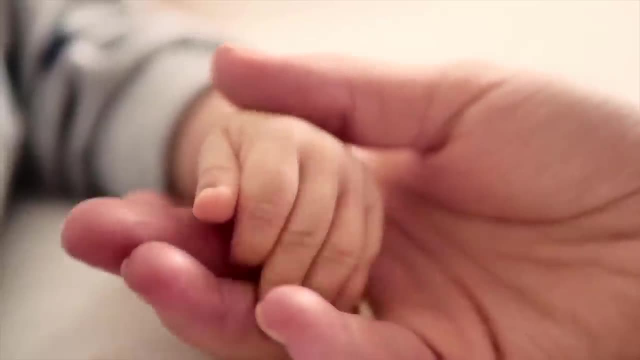 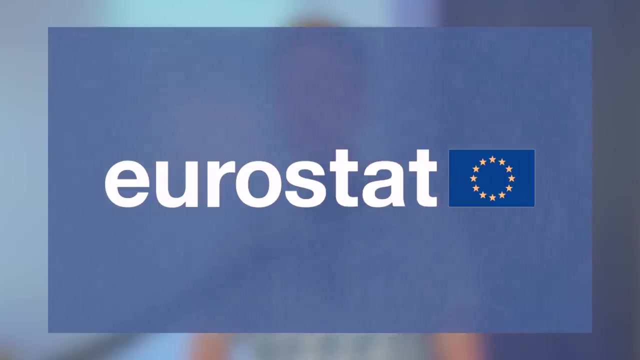 during the pandemic, when Europeans couldn't really have kids, And fertility rates have dropped precipitously, since Not all countries have released their data yet, which is why we don't have Eurostat data, But those that have saw steep declines. France, for example, has seen its 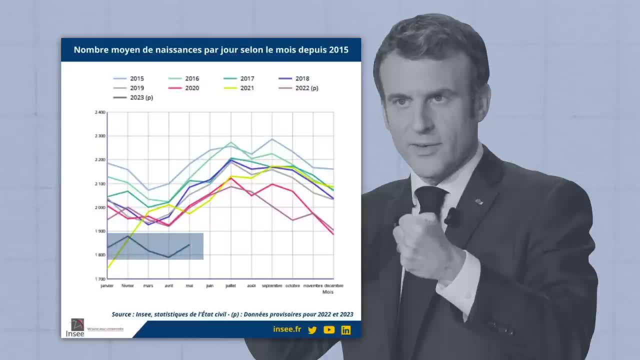 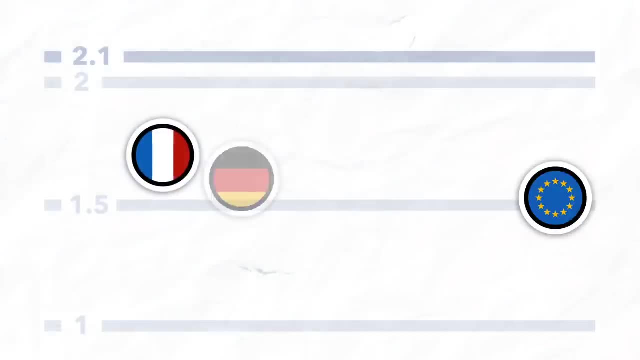 fertility rate fall by over 10%, With fewer babies so far in 2023 than ever before, which would imply a fertility rate of about 1.68.. Similarly, Germany's fertility rate fell from 1.58 in 2021 to 1.46 in 2022, and is expected to fall. 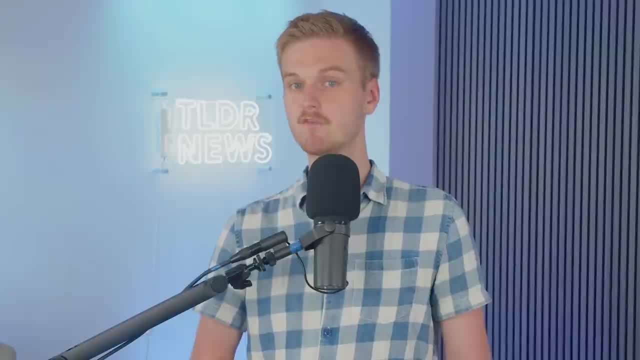 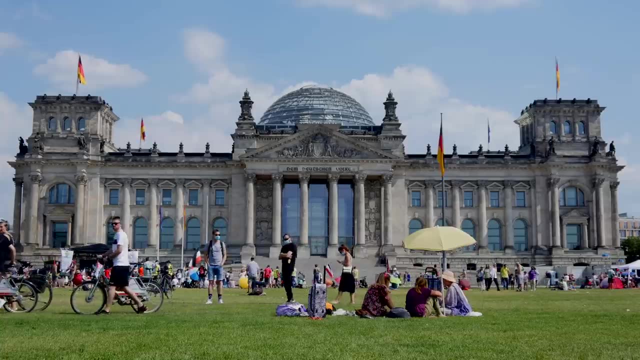 even further to 1.4 in 2023, driven by steep declines in German cities, Berlin and Munich, for example. both have fertility rates of about 1.2 at the moment. The Netherlands' fertility rate fell from 1.4 to 1.4 in 2022, but this is not the case for Australia. It is expected that the European 처mphtowns have a fertility rate of about 1.2 in 2022.. On top of that, the Netherlands' fertility rate fell 6.2 in 2021 to about 1.46 in 2023.. In fact, at least nine European countries, including Iceland. the Czech Republic, Albania, all the Nordics and all the Baltics are expected to see their fertility rates fall by at least 20% from 2021 to 2023. And many of the European countries with stable fertility rates are only avoiding decline because they're so low in the first place, Spain. 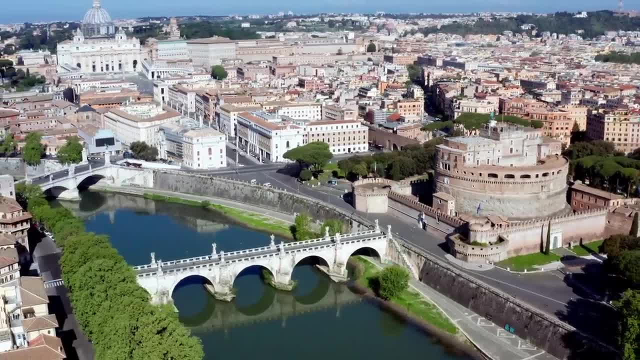 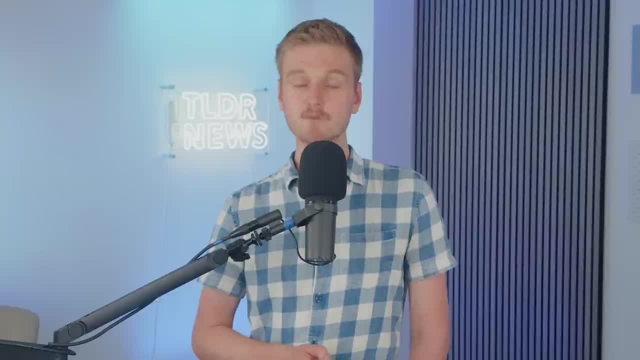 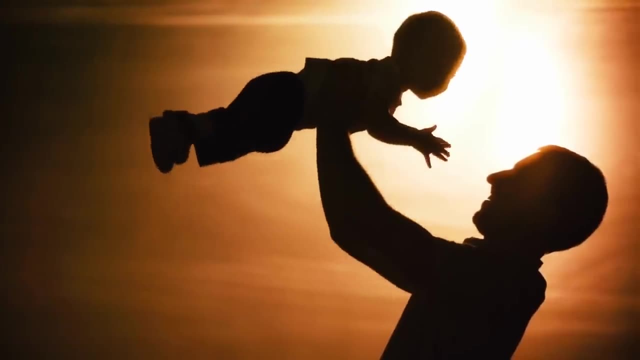 and Italy, for example, have relatively stable fertility rates, but they're both already well below the European average, at about 1.2 and 1.25 respectively. The problem has become so acute that many European governments have started implementing policies actively designed to increase their 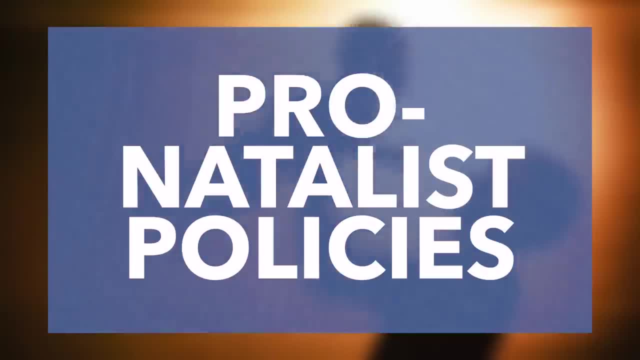 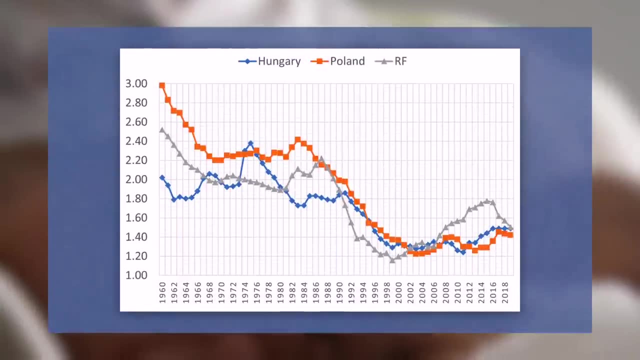 fertility rate, known as pro-natalist policies. Hungary and Poland first implemented pro-natalist policies in the 2000s, after their fertility rates collapsed in the 90s. Hungary now allows the European Union to implement pro-natalist policies in the 2000s. Hungary now allows the 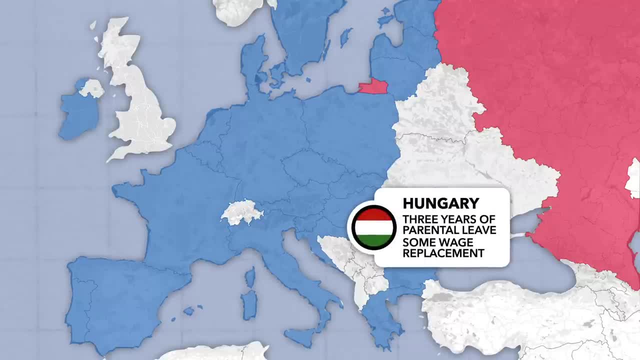 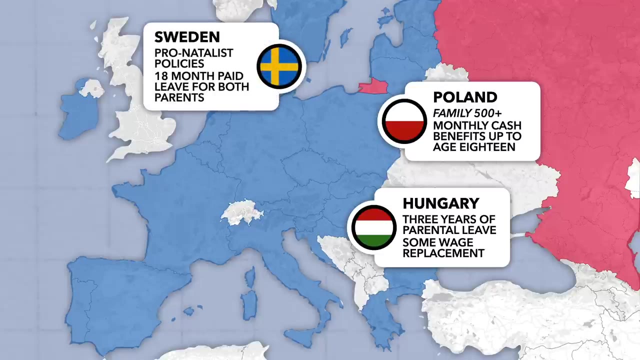 for a total of up to three years of paternal leave, with some wage replacement, And Poland's Family 500 Plus program provides a monthly cash benefit to all families for each child until the age of 18.. Sweden implemented tacitly pro-natalist policies in the early 2010s, including an 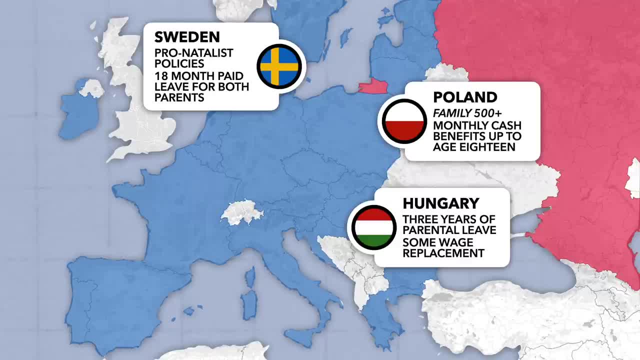 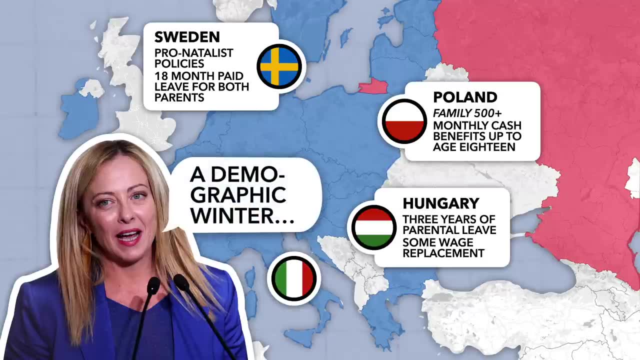 impressive 18 months of paid leave for each parent, And Georgia Maloney has been actively trying to boost birth rates in Italy, railing against what she's described as the demographic winter. Worryingly for all these politicians, history suggests that it's very hard to reverse. 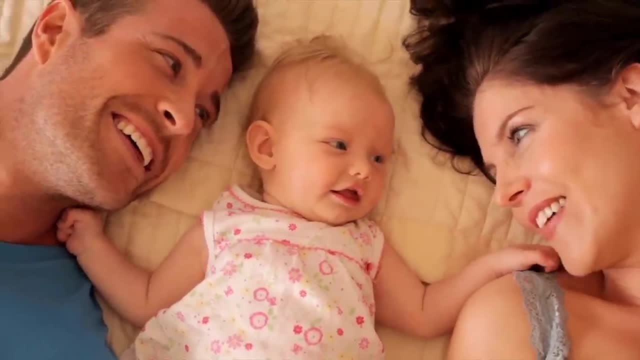 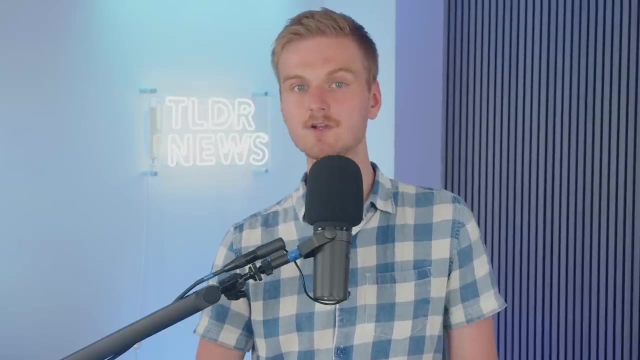 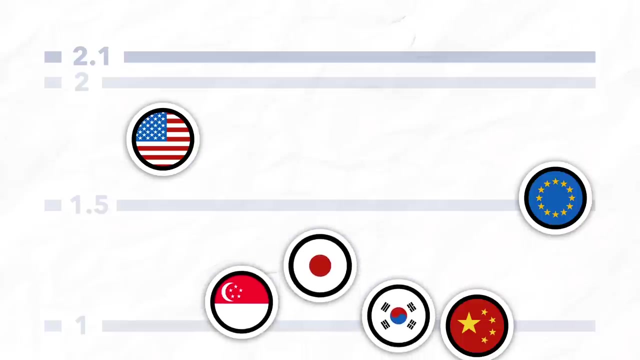 demographic decline. Despite their generous pro-family policies, fertility rates are still below replacement rates in all the countries we just mentioned, And decades of pro-natalist policymaking have done little to stem the demographic decline in South Korea, Singapore and Japan. The most obvious solution is immigration, especially of young people. 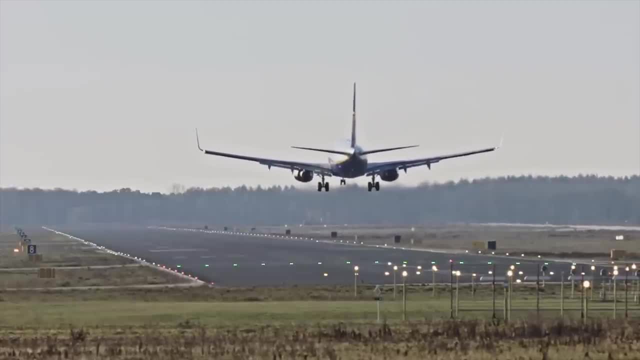 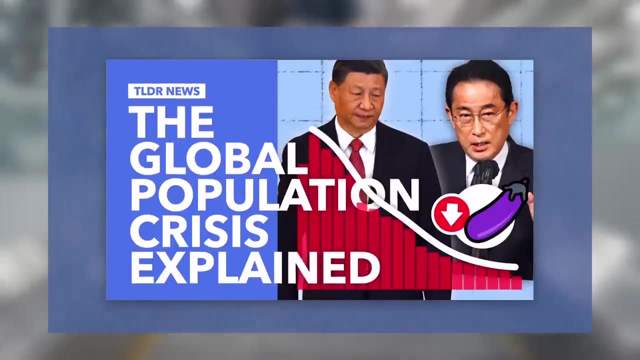 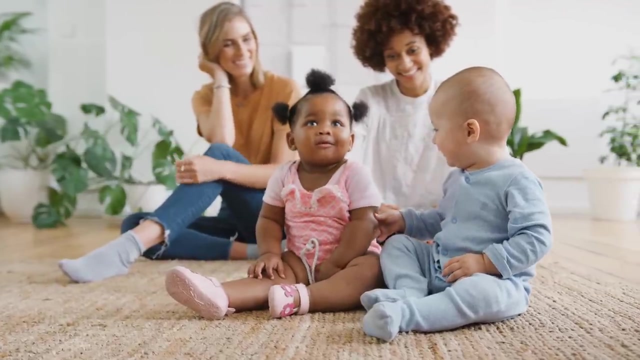 But this has proved increasingly controversial in Europe, and even then it's not clear that this is a sustainable solution, Both because fertility rates in the rest of the world are also falling fast and because, after at most a couple of generations, immigrants usually end up converging to their new country's fertility rates. 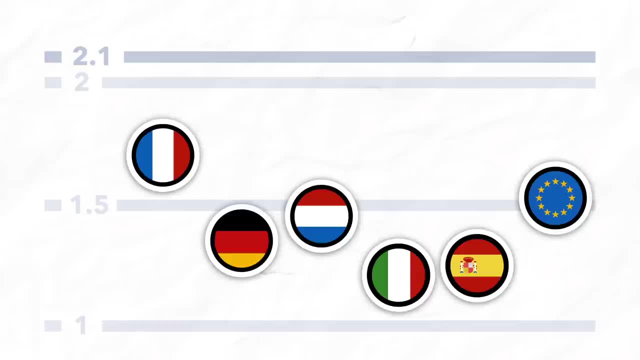 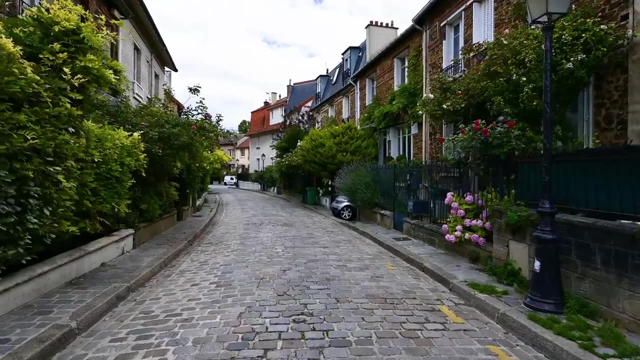 If governments are serious about reversing Europe's demographic decline, however, then they should start by looking at housing. There's good evidence that expensive housing isn't helping. In general, expensive housing means more young adults still live at home, and there is a lot of evidence that expensive housing is not helping.